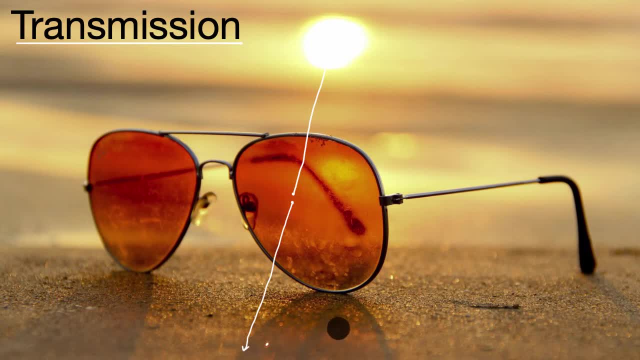 of transmission and what gets transmitted is dependent on the wavelengths of the wave, In this case the wavelengths of light, and also about the material that they are going through. So, for example, these sunglasses right over here, many sunglasses try to keep out UV light, ultraviolet light. 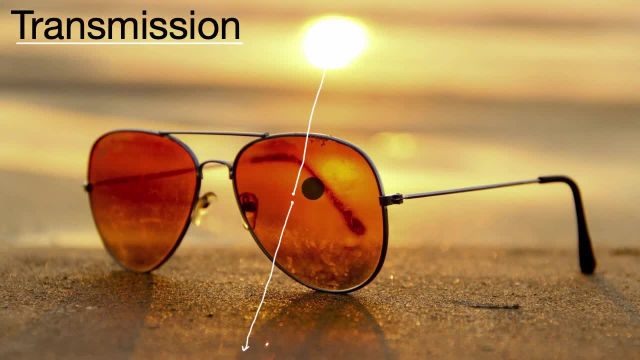 which is a higher frequency than visible light. but that's what causes sunburns And that can also damage your eyes. So those high frequencies are not making it through. And we could also see that this sunglass right over here. it kind of has an orangish color. 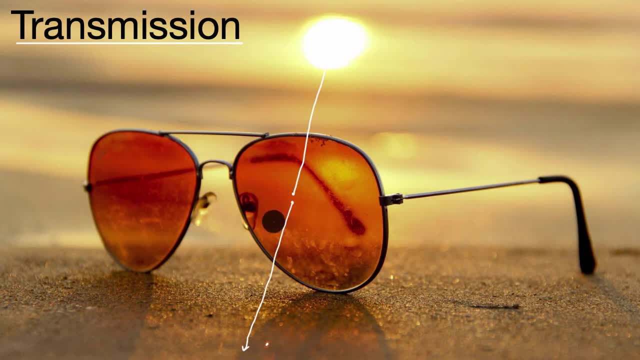 which means that things that are closer to that end of the spectrum, closer to the red, the oranges and the yellows, are getting through, which means that it's filtering out blue light, So the blue light isn't getting transmitted through as much. 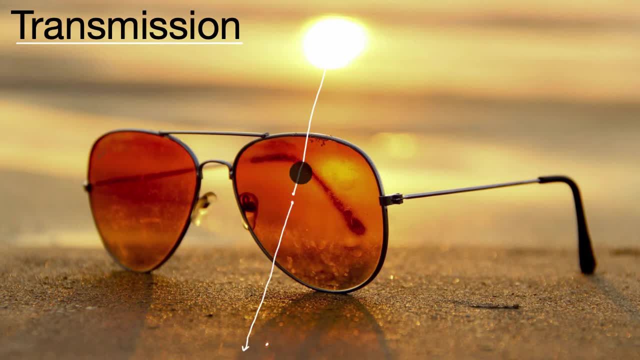 as say, the red, orange and yellow light, And that's why we see this as red, orange or yellow. And then, of course, the light will get to that sand particle- Now transmission, as I mentioned, will get to that sand particle, Now transmission, as I mentioned. 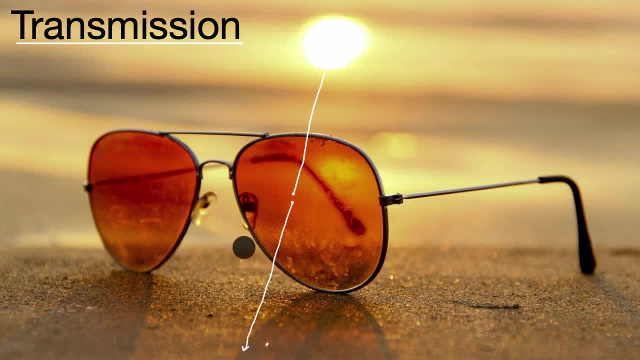 it isn't just about light waves. We could talk about one of our other favorite types of waves, for example, sound waves. If you are in a room, you have probably experienced the fact that, even if you were to close the door- and I do this a lot- 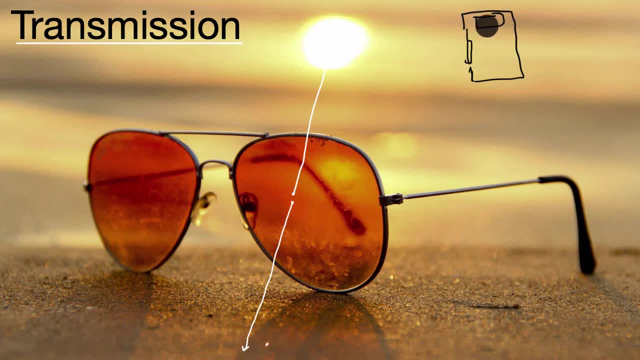 because I record a lot of videos. This is me in my little closet recording a video. This is a top view of what I'm doing right now. A lot of times my kids are in other parts of the house and they're making a lot of noise. 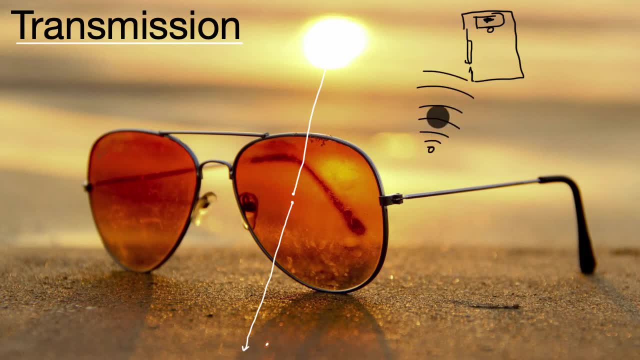 And, as we've talked about, sound waves are nothing but traveling pressure waves through the air. Those air particles are knocking one into another, But in order to make it to me, they need to get through that wall, And the way they do that is they get transmitted. 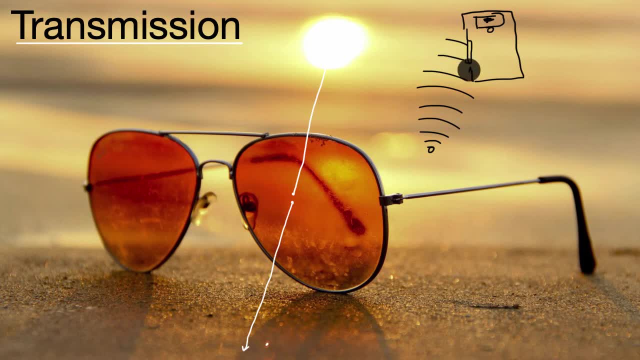 to through that wall. So those air particles make the particles or make the atoms or the molecules in the wall start vibrating, They bump into each other And then the particles on the other side of the wall will bump into the air in my little closet. 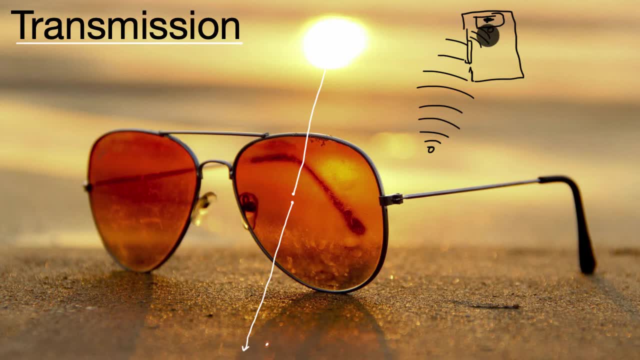 And then we will have once again the sound waves. make it to me Now the overall magnitude of the sound. the volume of the sound will likely be diminished, And not all of the frequencies of the sound will be transmitted equally. Different frequencies of sound waves.